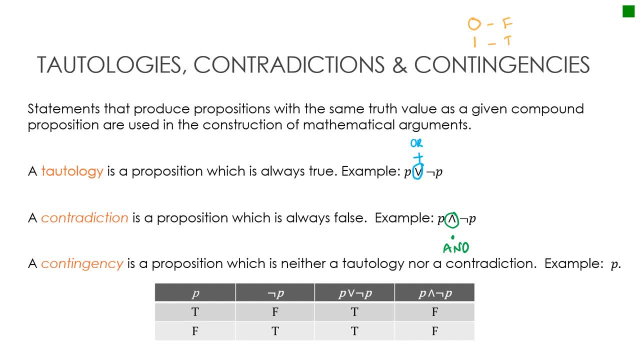 about together in just a minute, But essentially what I could have done instead of writing: true, here is right one. and for false right, zero. and for false right, zero and true right one, Then this is one and one and this is zero and zero. And, as you can see, I didn't really change anything, I just 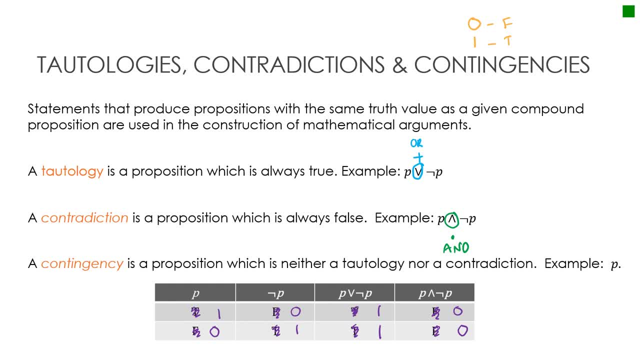 changed the format. I substituted one value in for it. Now, the reason I bring this up is not only will you possibly see it if you're looking at other videos, but also that we can use it in examples like this. So, if you're ever unsure if I'm looking, 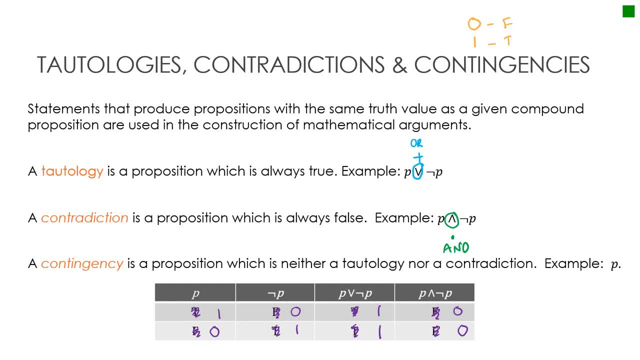 at P or not P, then let's take a look down here. I can think of this as a math problem That says, well, if P is true, that's one, And then the or is zero, And if P is true, then not P is. 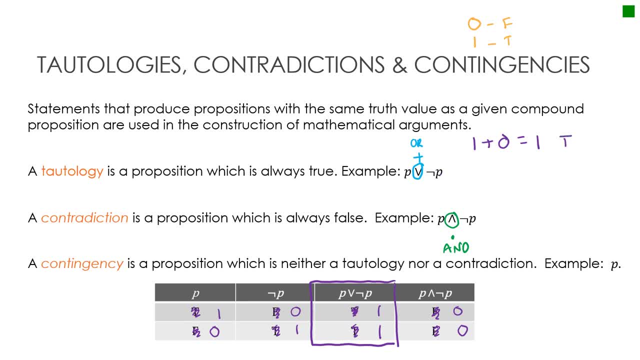 false And that adds up to one, And we all know one means true. Or let's say P were false, So that would be zero, Then not P would be true, And if I add those together I get one And that is true. 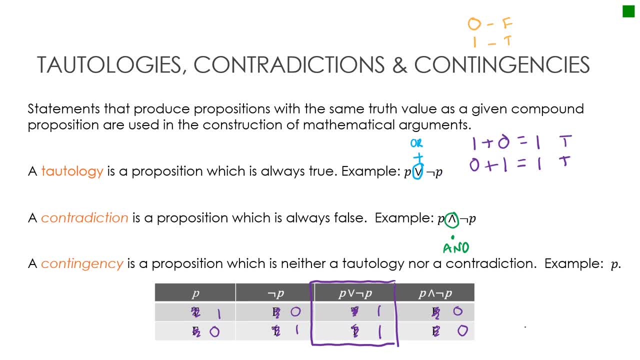 And that is this column. Oops, That is this column Right here Now. this is considered a tautology because, as we can see, this is true No matter what's happening over here. I get two ones or two trues. So that is a tautology, Always true. 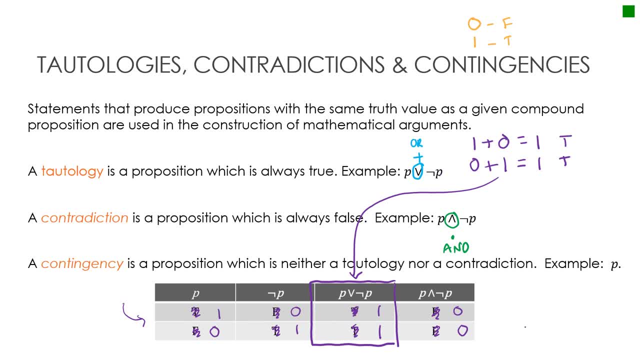 Now let's look at the contradiction. So a contradiction is a proposition which is always false. So before we look at the truth table, let's look at the math. Same thing here. Let's say P is true, So that's one. 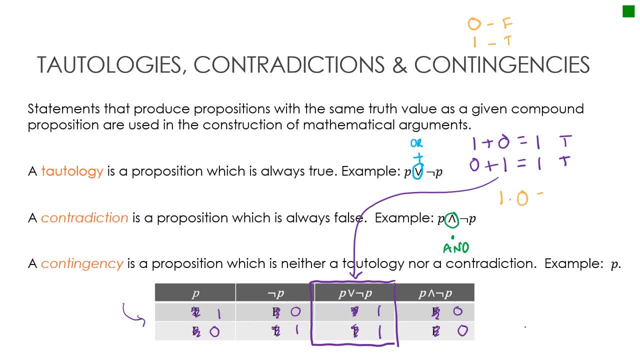 Then not P is false And that's zero. And if I multiply them I get zero, And zero means false. Or let's say P was false, which means not P is true, And if I multiply them I get zero, which 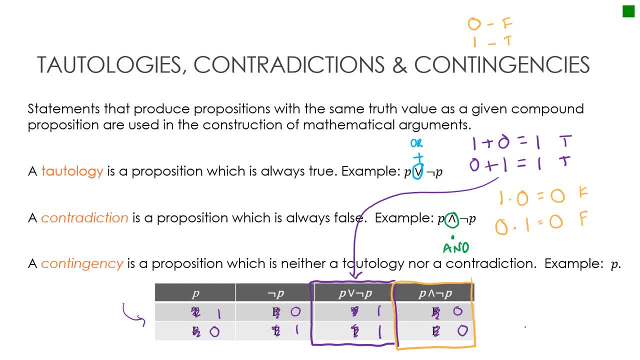 means false. So, as we can see, P and not P is always false and therefore a contradiction. So what does any of that mean? Well, we want to look at the contradiction. So let's look at the contradiction. So let's look at the. 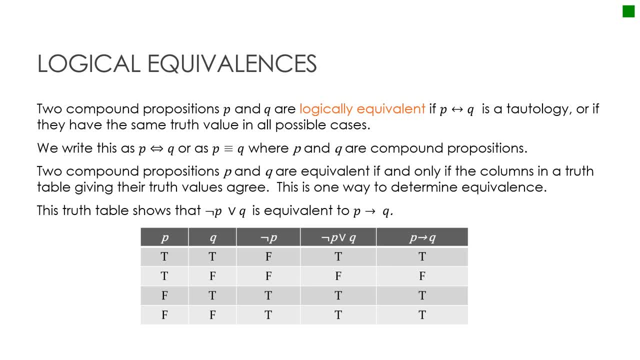 刚 ca me cgiäk gain Network propositions that are logically equivalent. and they're logically equivalent if P, if and only if Q is a tautology, which basically means if I can do a truth table and show that the truth table is the same for both propositions, then it is logically equivalent. So I want you to note. this group. we're learning now. The numbers that we keep to remember are all different here, so we'll just submit more. for me to analyze our improvement on the product here. This shows something we've already learned, So it is even more. And here it's printable, So there are 다양한 ways for us to perform. 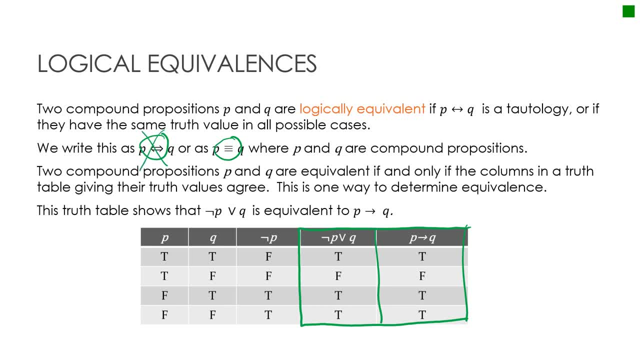 predictions, But that does give us a malicious response. That means pushing forward. So instead of thinking we will use Typically, we don't use this one. You won't see that very often, but you will see the equivalent sign, the three equal sign, which is equivalent And essentially what we're looking. 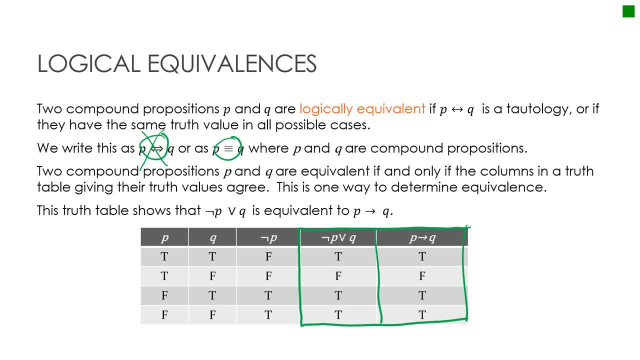 for, as I said, is the columns of the truth table having the exact same values, And so I've already worked this one out for you, just so that you could see. but obviously we all remember how to find these two columns. We take whatever our propositions are and write them all out. 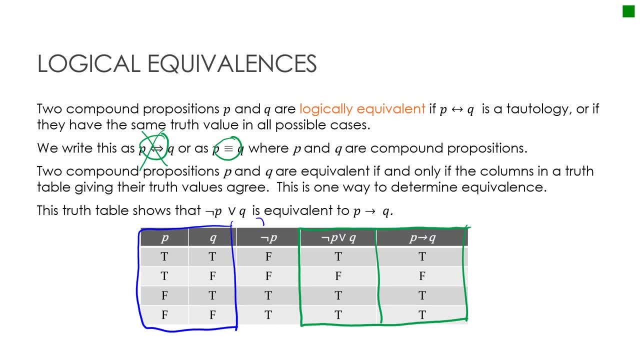 And then I knew that I was using a, not p, as part of one of my- excuse me, one of my propositions. And then I just went through and filled these out And notice I get false, true, true, true, which again, if you feel better, using one, zero, one, one, one, zero, one one. 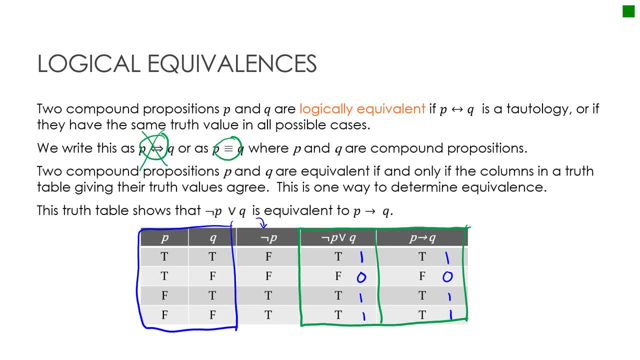 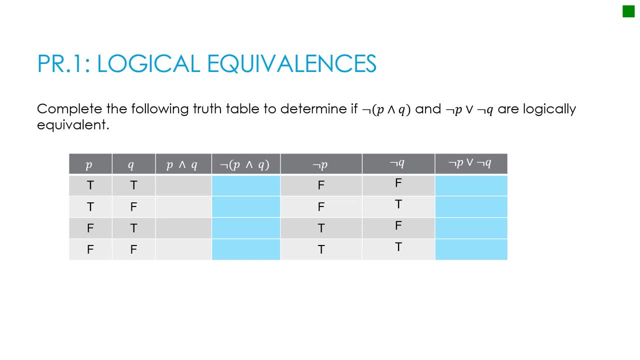 that is just fine by me. What I would like you to do is take a look at my propositional statements. not P and Q, and not P or not Q. I want to show that those two things are logically equivalent, essentially that those are saying the. 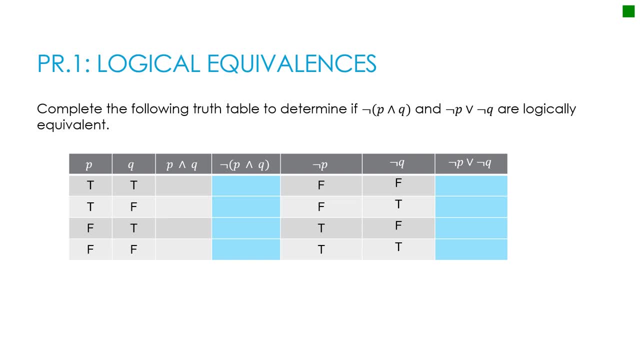 same thing. So press pause, try filling in all of the parts. Obviously, the blue parts are the parts that we want to show, are logically equivalent, and then, once you are done, press play to see how you did. So let's see how we can do together. I. 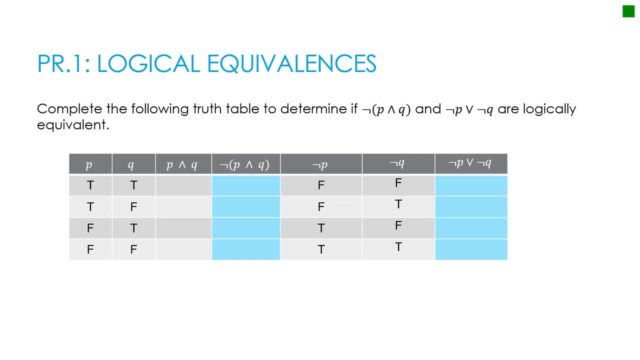 have P, I have Q and notice I've set up the first one as P and Q. So P and Q is true. So if I take a look at my propositional statement I'll see that they are both true. So that would be here, but not here, and not here and not here. The next. 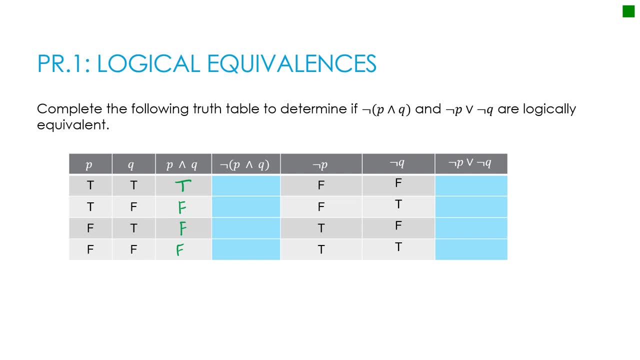 column is the negation of that statement, which gives me false, true, true, true. So I took these and I negated them. I changed the sign. The next one is not P or Q. So if I take a look at my propositional statement and notice I've. 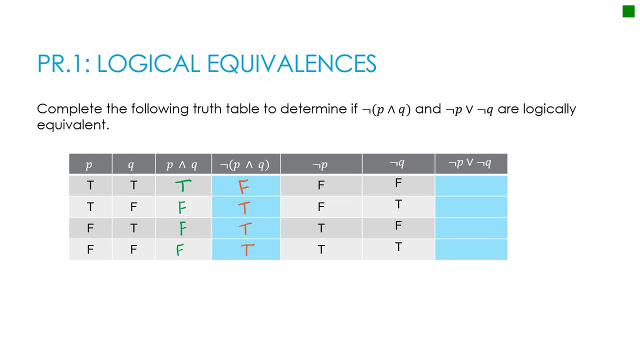 not Q, which means I just need one of them to be true. so this is false because they're both false. this one is true because, as I can see, I have a true, this one is true because I have a true and this one is true because I have a couple. 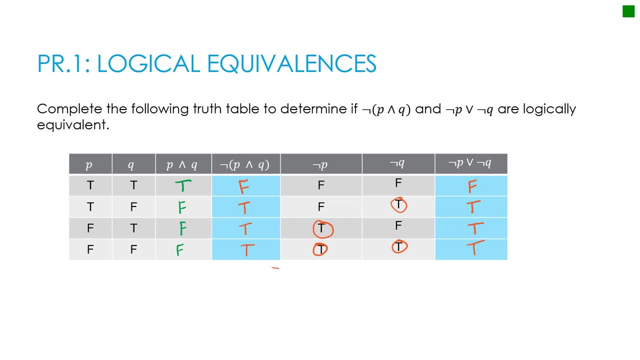 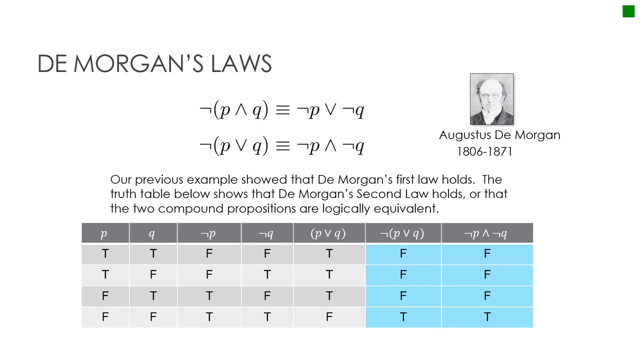 of truths, and what I notice here is that I have just shown that these two statements are equivalent. so essentially, what you just did, without even knowing it, is, you proved De Morgan's first law. the first law says: if you have the negation of a conjunction, it is equivalent to the disjunction of the negation of each of those phrases. so 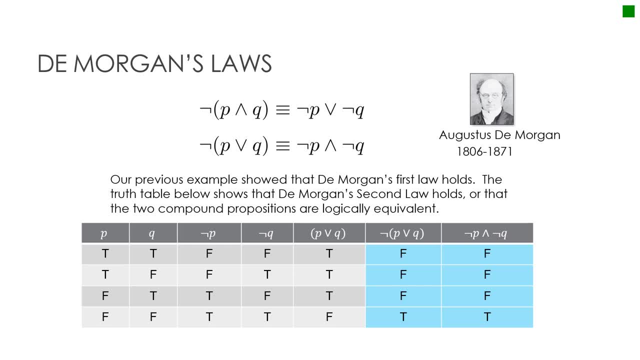 it's kind of like we're distributing the negation, but in doing so the conjunction turns into the negation of each of those phrases. so essentially what you just did turns into a disjunction. De Morgan's second law is kind of the opposite of that. we're saying: if we have a negation of a disjunction, that's equivalent to 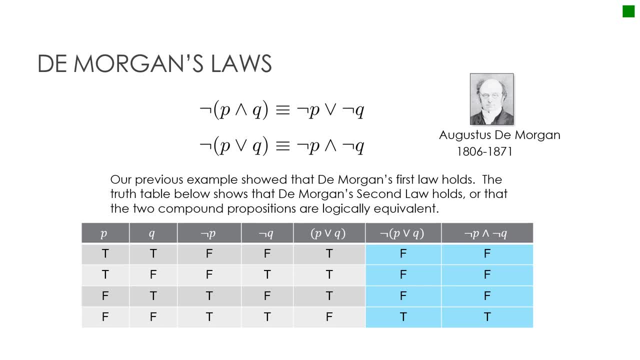 the conjunction of the negation of each of those propositional statements. so again, just note that each time if it's a conjunction it turns into a disjunction, and vice versa. so that basically says, yeah, I have the answer and I'm gonna purchase it back again. these two, Legra is the normal conductor again. these two laws are super. 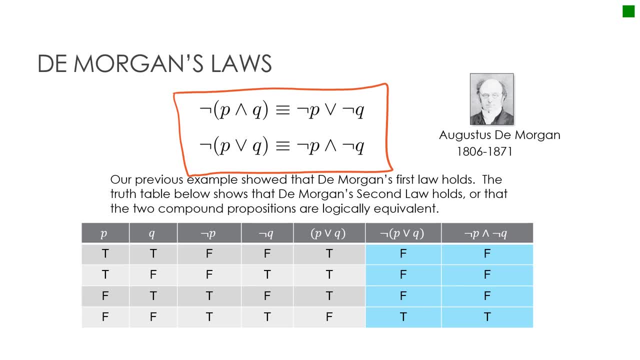 duper, duper, important. yes, that was a duper twice. people, you are gonna use these all of the time, so please make sure that you just remember them. write them somewhere that are easy to get to. now, obviously, excuse me, obviously you can see below that I have done the truth. 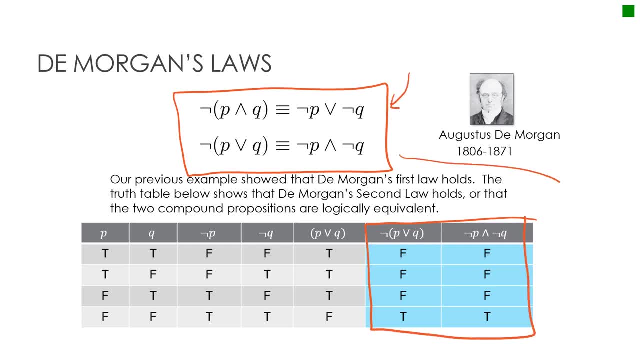 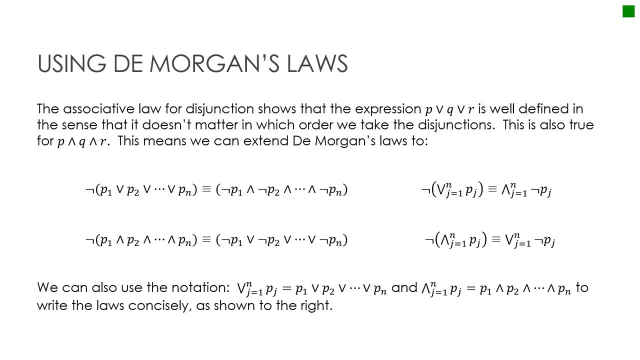 table for you that shows that these two things are in fact equivalent. so we did right down here, showing that they are in fact equivalent. We just talked about De Morgan's law for two propositions, but I want you to notice that it is the same idea no matter how many propositions we have. So in my first example here I have 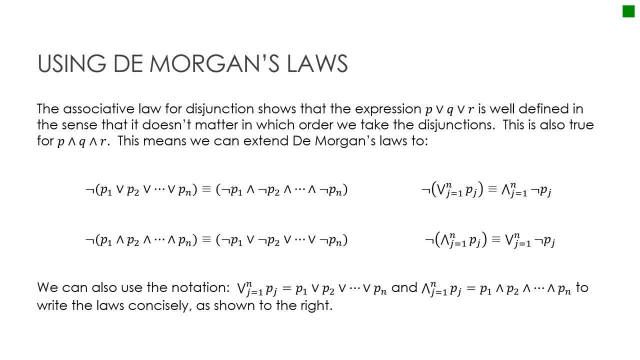 the negation of a disjunction. and it doesn't matter how many of these separate propositions I have, The same quality holds true. I'm essentially negating each proposition and then taking the conjunction, And same thing for the other law that says: hey, if we have a negation of the conjunction, then 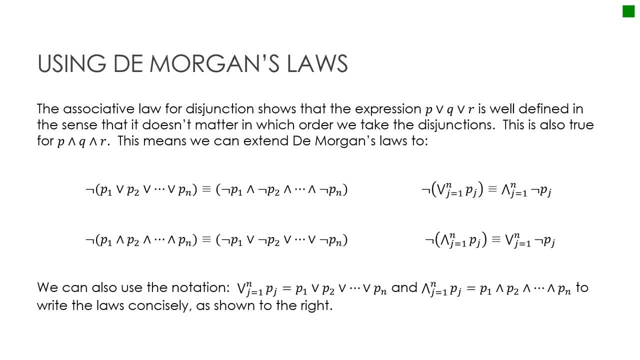 it's the disjunction of each of the negated propositions. The other thing I wanted to point out is this other way, a bit more concise way, that we can write something as ridiculous as this, in the same way that we would use a summation formula, where we can write things a little bit more concisely in, say, calculus. 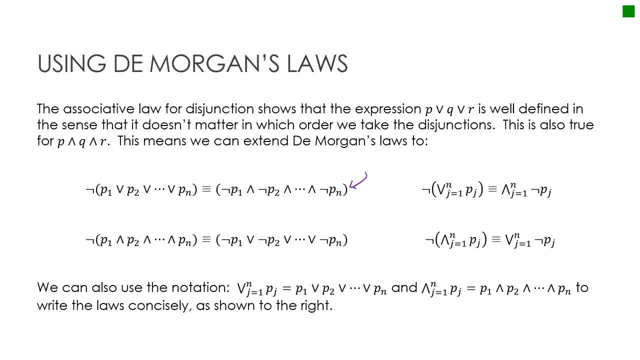 That is the same idea here. So here I'm saying I'm negating the disjunction of each of these values and that's the same as the conjunction of the negation of each of those values, etc. So just some more notation that you might come across. 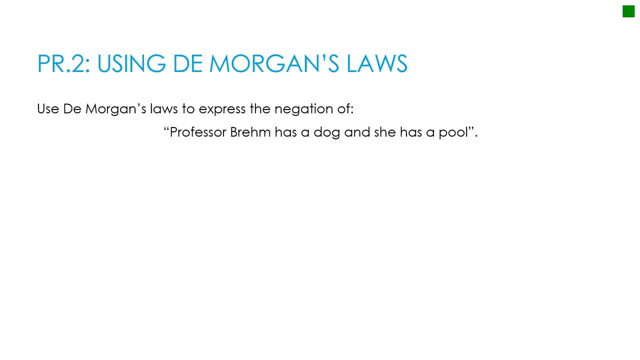 So we haven't done one of these together, but I feel confident that you can do it. I would like for you to use DeMorgan's laws to express the negation of Professor Brame- that's me has a dog and she has a pool. 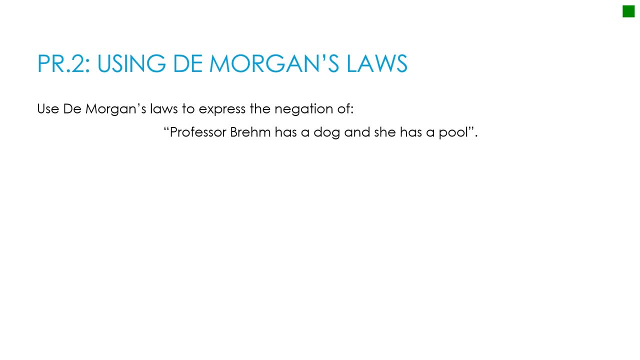 So first thing, obviously, that you would want to do is write the propositions And if this is an and or an, or a conjunction, disjunction etc. and then use DeMorgan's law to negate it. So give that a shot, press pause, give it a shot, then press play to see how you did. 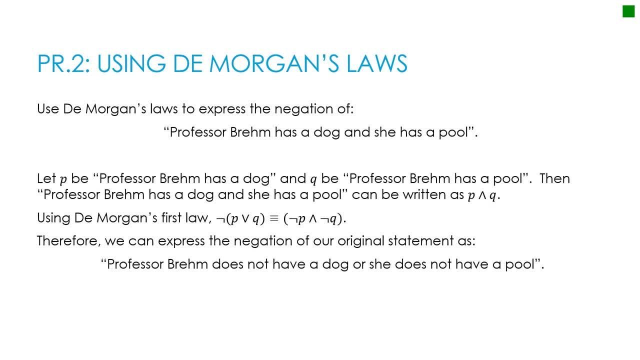 So, again, the first thing that you have to do- and you really have to do it- is you have to assign Professor Brame has a dog as P, Professor Brame has a pool As Q And then write the original statement using that P and Q. 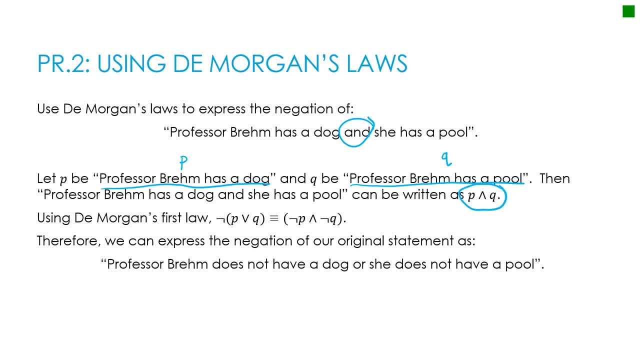 And because this is an, and I can write that as the conjunction of P and Q, Then again, using DeMorgan's first law, if I'm trying to negate, the negation of a conjunction is the disjunction of the negations. 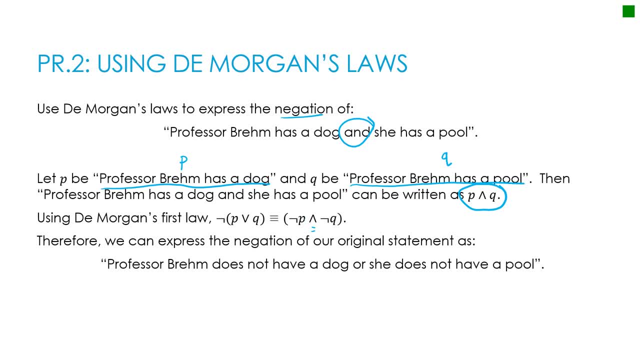 So I'm going to negate P, Which is: Professor Brame does not have a dog. I'm going to negate Q- Professor Brame does not have a pool- And instead I'm now using my: or. So Professor Brame does not have a dog or she does not have a pool. 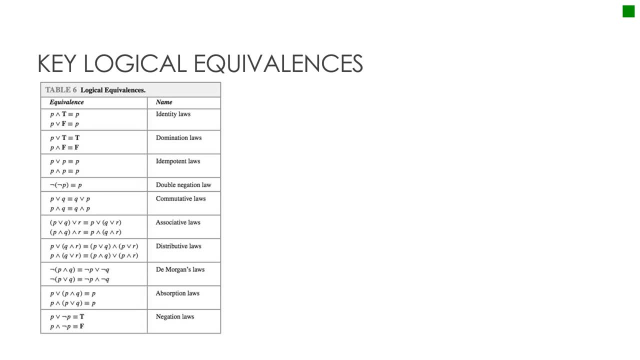 Over this slide and the next slide. we're going to look at some key logical equivalences. I suggest that you print out the slides or make yourself a cheat sheet just as a way to easily reference all of these. I don't expect you to have them memorized, but you do need to be familiar with them. 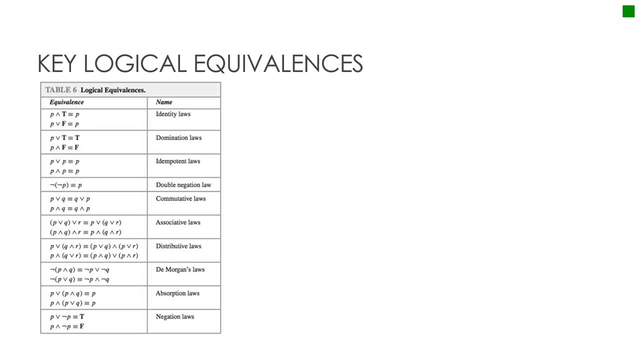 So you sort of have that arsenal as we're working through proving logical equivalences. Now, I'm not going to go through each and every one of these, but I do just want to, you know, show a few of them to you or how they work. 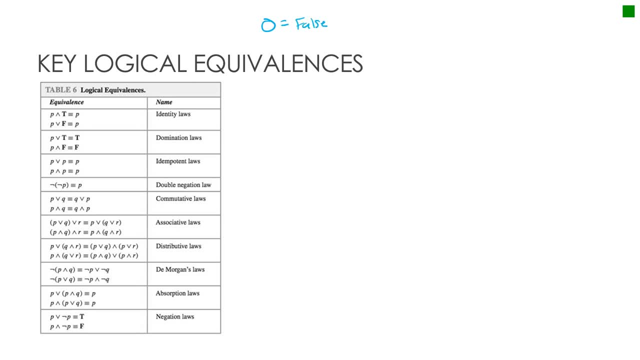 Keeping in mind that we use zero for false and we use one for true. That's sort of a strategy as you're looking at these. If you're not quite sure if you're doing it right, Maybe try using the plus or the multiplication with zero and one and make it make a little bit more sense. 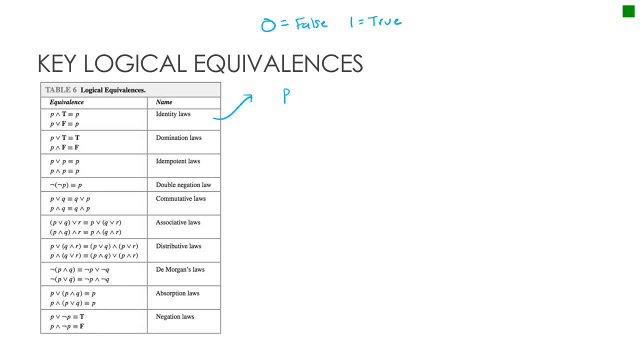 So, for instance, let's take a look at that first identity law that says P and true is equivalent to P. Now, why does this work? Well, let's say P were true And one is true. Then I'm going to get an answer of one. 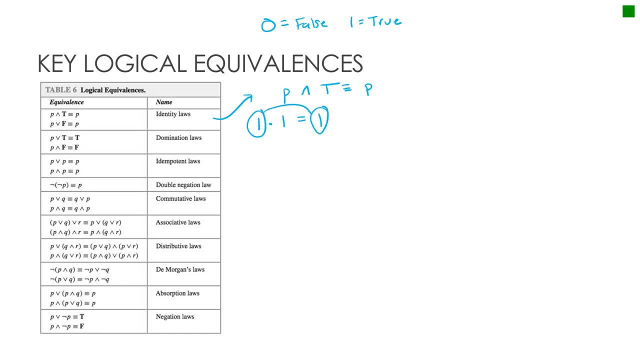 And, as we can see, These two are equivalent. Let's say P were false And I'm still taking it times one for true. Then I get zero and I can see that these two are equivalent. So if I have a true, it holds that P, that we can just replace that with P. 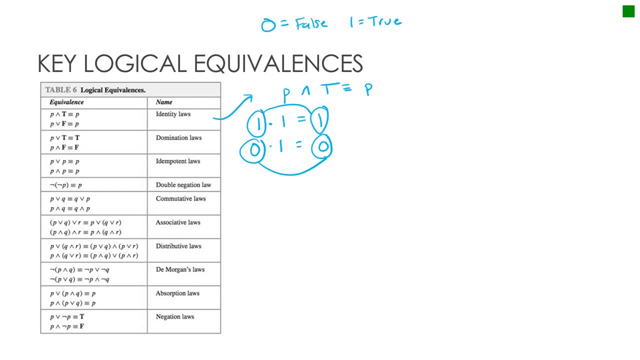 You can do the same thing for the other identity law, The domination laws. again, pretty straightforward. If I have P or true, I know in an or statement that all I need is one of the two to be true And therefore, since this one is true, then the whole statement is true. 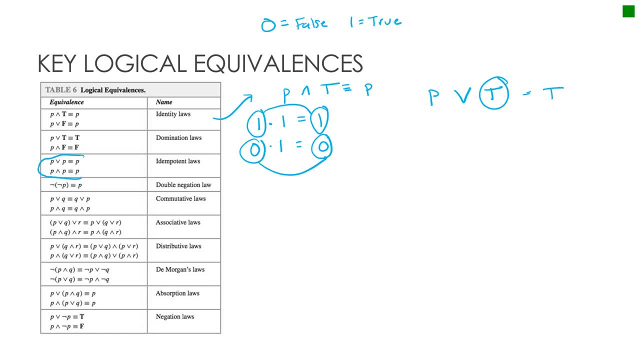 Same thing for the other one. These are kind of fun. Just remember that you're always going to end up with P Double negation law. Two wrongs make a right, but only in mathematics. Commutative and associative laws, Just like the commutative law for addition and multiplication. 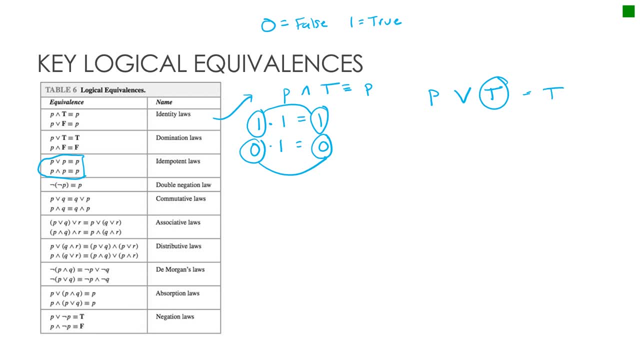 Same thing holds true for our logical equivalences, The distributive law as well. Notice, I'm just going to distribute that P to both values inside. So again, that's a strategy you're going to use quite often. De Morgan's laws are we already talked about. 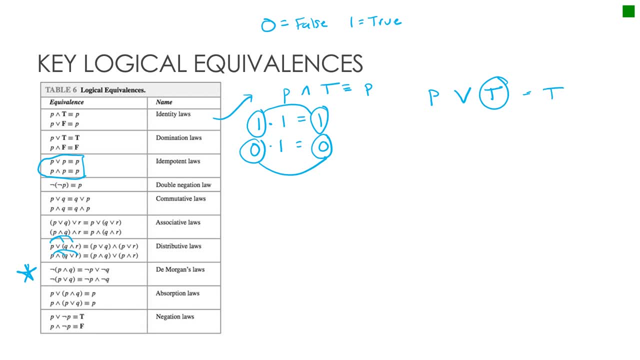 These are super important. We're going to use them all the time. The absorption law: Let's say I have P or P and Q And I'm saying it's equivalent to P, So why does it work that way? Well, let's see. 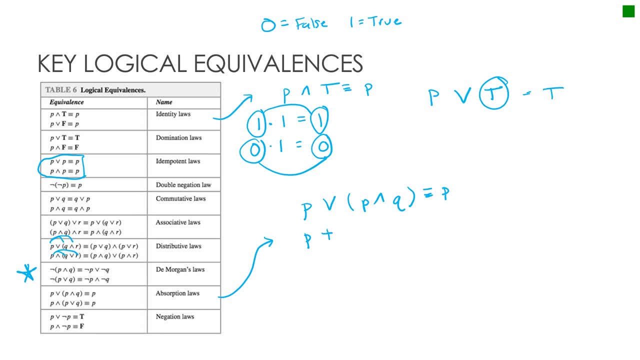 I've got. let's write this as P or P times Q, Which means I could really write this as P: 1 plus Q. Well, 1 plus Q is saying essentially true plus Q, Which is true. So basically I have P times true. 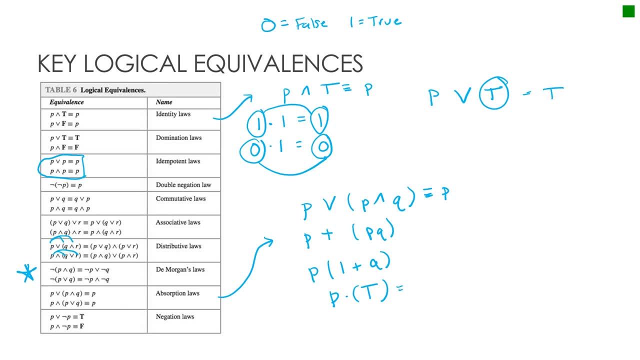 And, as we can see, P times- true is going to be P, Because we already talked about that right up here. So absorption law, maybe not as easy as the others, but pretty straightforward. And then the negation law, And this again is pretty straightforward. 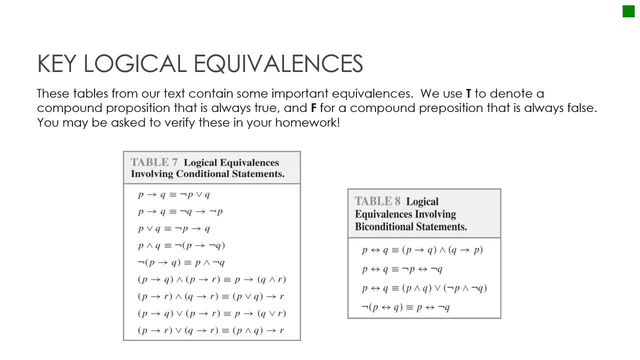 So take some time to look over those. And here are the other logical equivalences, And so, as you can see, we've got quite a few other things that we can take a look at. Again, I encourage you to make yourself a reference sheet or print off these slides. 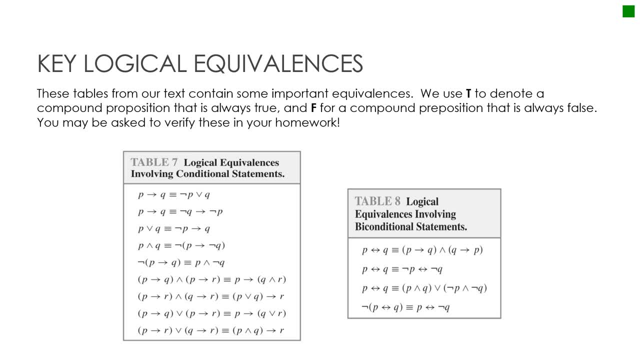 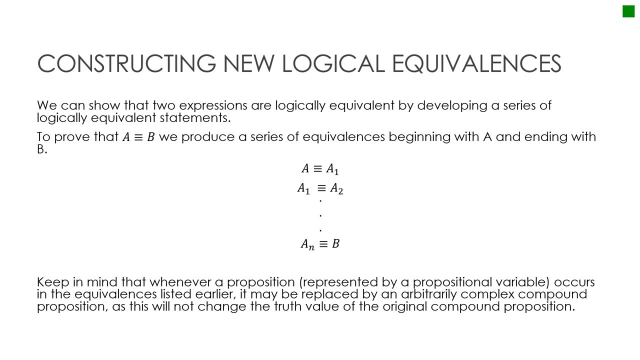 I'm not going to go through each of these. I'll leave that for you to do on your own. So what does all of that mean? It means that we can show that two expressions are logically equivalent by basically developing a series of equivalent statements. 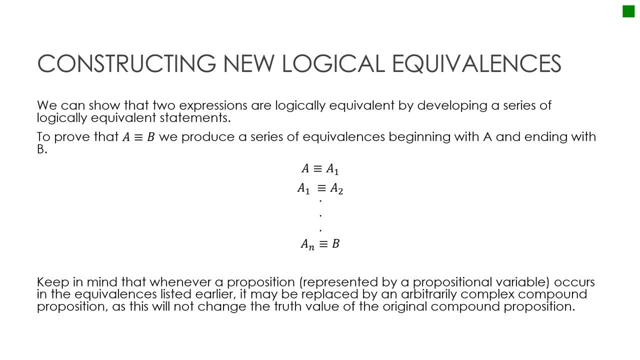 Where are those statements going to come from, All of those properties that we just talked about? So, essentially, I'm saying, if I want to prove that A is equivalent to B, I'm going to prove A is equivalent to something, That that something is equivalent to something else. 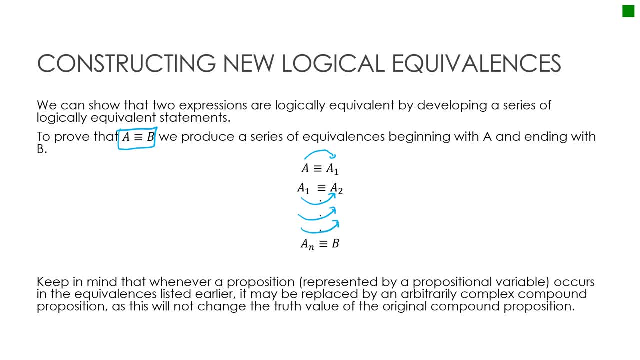 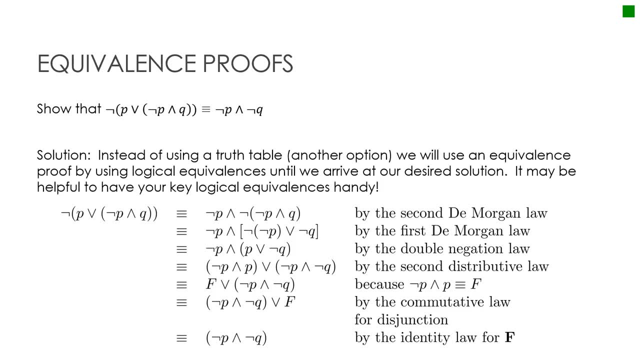 And that's equivalent to something else, And that's equivalent to something else until I finally arrive at B. So this obviously makes so much more sense when you can actually see it in action or see what's going on. So this is kind of like going back to geometry, where you did sort of a two column proof. 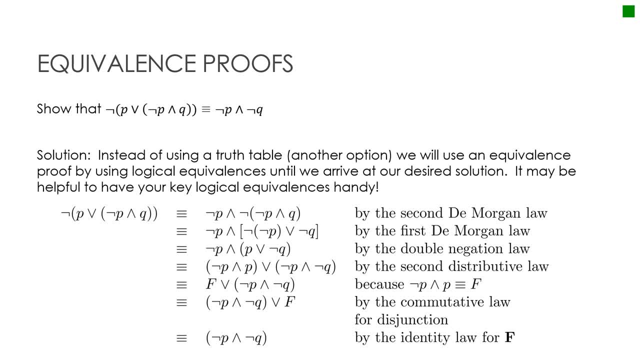 You said: here's what's happening. Here's the law that I'm using that says it's okay for me to do this. So here is the statement that we are trying to prove equivalence with And, again, this is an equivalence proof. 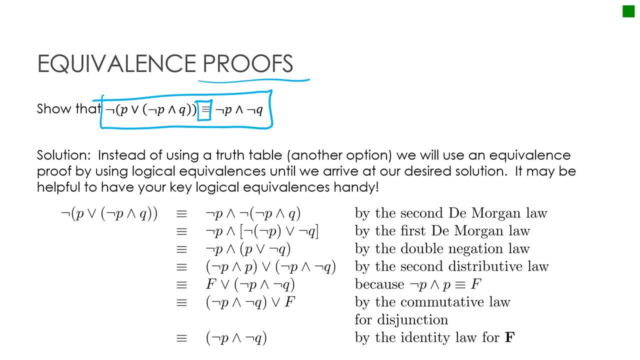 So we could use a truth table. We're familiar with truth tables, We just talked about them a little bit ago. That's certainly an option, But instead let's look at an equivalence proof, And in an equivalence proof, I'm going to start with the first part, or the first propositional phrase. 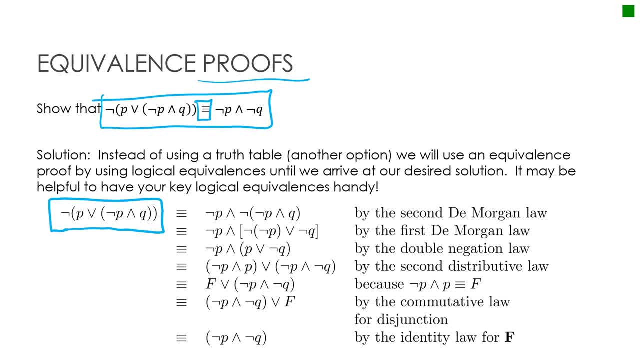 And I'm going to prove its equivalence essentially by applying some of the rules and laws that we just talked about. So let's begin. Remember my end goal is not P and not Q. I want to prove that that is equivalent to something else. 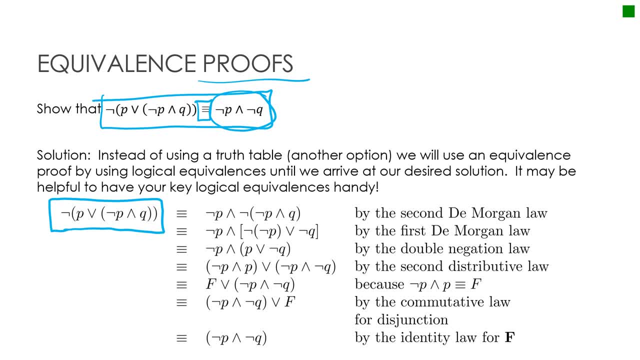 That is equivalent to what I'm starting with, which is the negation of the disjunction of P and not P and Q. So first thing I can do- because I have the negation of this whole thing here- is I can negate each term, but turn it from a disjunction into a conjunction. 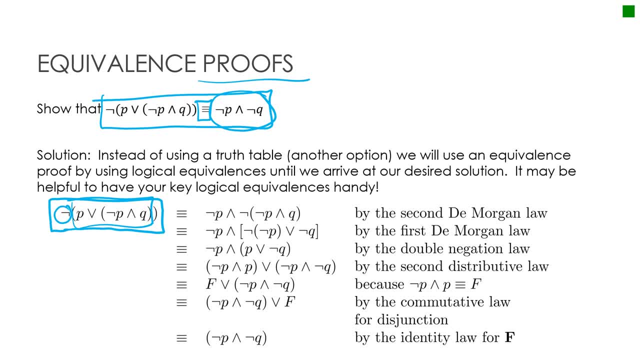 And again, that's just using De Morgan's Law. And notice it says De Morgan's Law, De Morgan's Second Law, De Morgan's First Law, Whatever Just put De Morgan there. so I know that you know that's where it came from. 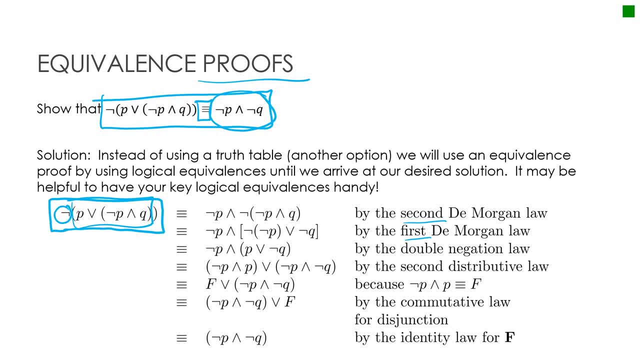 And then I'm going to use De Morgan's again, but in a different way, Because, as we can see, I still have the same idea. I've got the negation, this time of a conjunction And I'm going to turn that into the disjunction of the negation of each of those propositions. 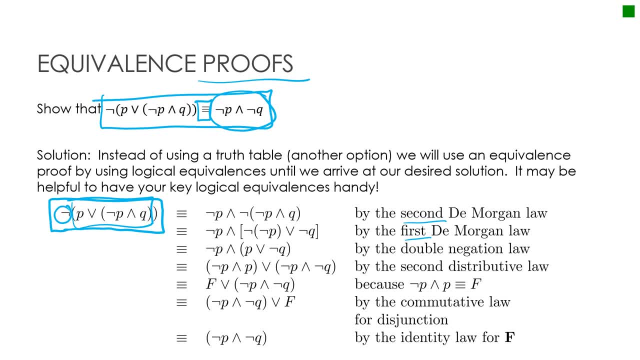 So that is again the first De Morgan's Law. And then I see that I've got two negatives. so I'm using the double negation law for two wrongs making a right. And then I'm looking at distributing. This is a distributive property where I can distribute the not P to both of those terms. 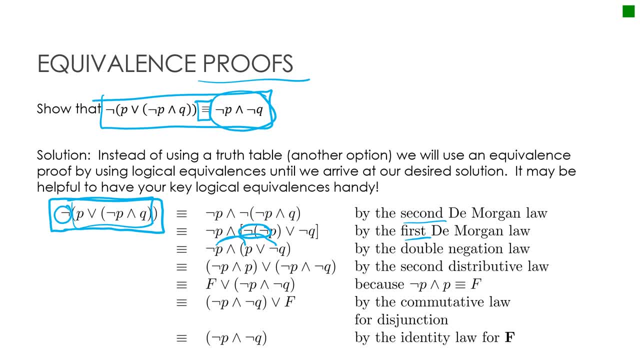 Notice, to just make sure you keep straight that this symbol is here. This one is still in the middle. Same way with normal distributive property. but sometimes you can get confused, since we don't have pluses and multiplication signs etc. Now, looking at this, not P and P. we know that that is always false. 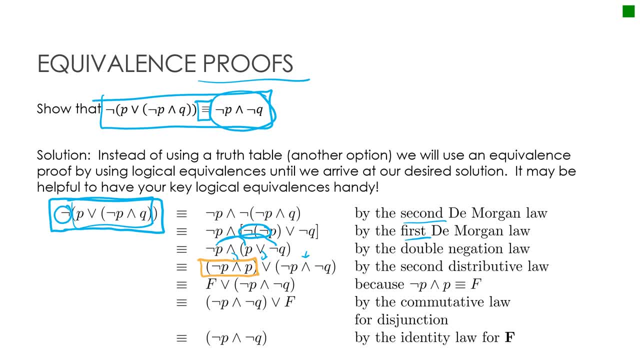 That is always false because we need both to be true and that's impossible And therefore that is false. And then I'm saying let's use the commutative law to basically switch the order, Because I want the F to come second. 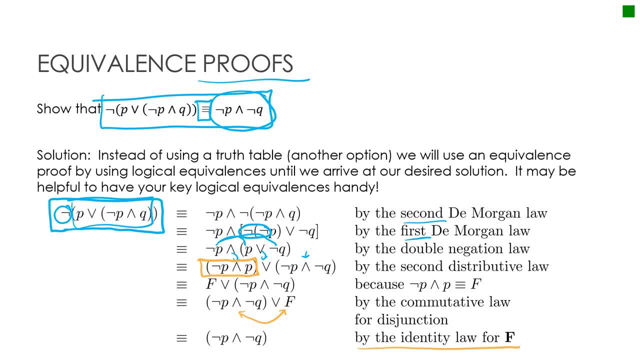 And then I'm using the identity law, And the identity law says- because this is an or and this is a false- that my value is going to be whatever the not P and not Q was, And therefore I ended up where I wanted to right here. 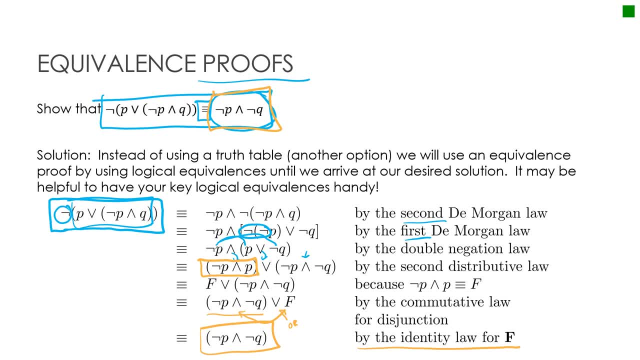 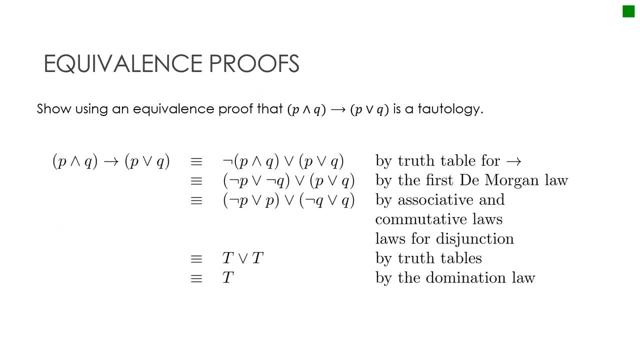 So that is an equivalence proof. I'm using laws and stating what those laws were to end up at my required destination. Here's another for us to try together. And again, notice that I've just put all of the answers out here for you so that I'm not showing them a little bit at a time. 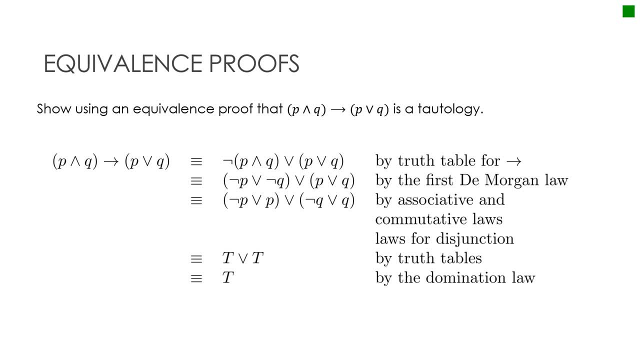 And that is so that you can sort of understand without having to feel like you're writing things down. But let's take a look at it a little bit at a time. So essentially it's saying: prove that all of this is a tautology. 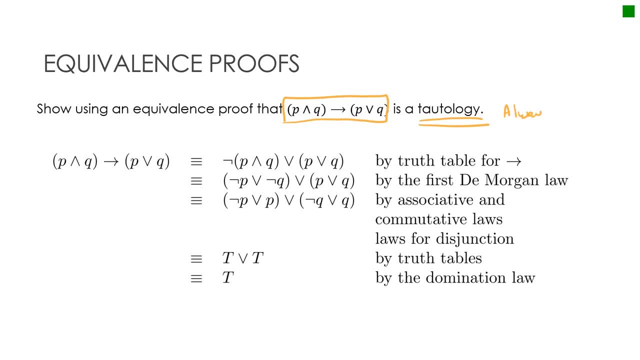 And remember, in a tautology we're saying: it's always true. So essentially, we're proving that this is true, This is always true. So, looking at all of the different tools that we have in our equivalence proof toolbox, we're starting here. 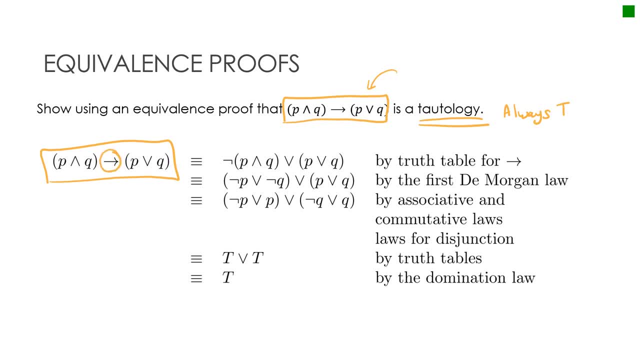 And the first thing I'm doing is I'm saying this is an if-then And I've got a property that says if you have an if-then, you can turn that into a disjunction of the negation of the first compound proposition. 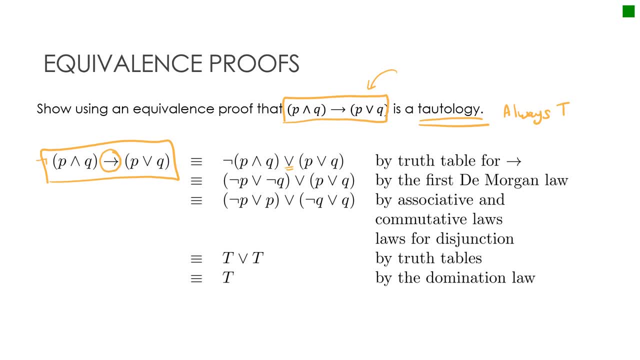 And then just keep the second one exactly as it was. So notice, I've just used the truth table for the if-then I think there's another rule, another name for that rule, but I don't recall it off the top of my head. 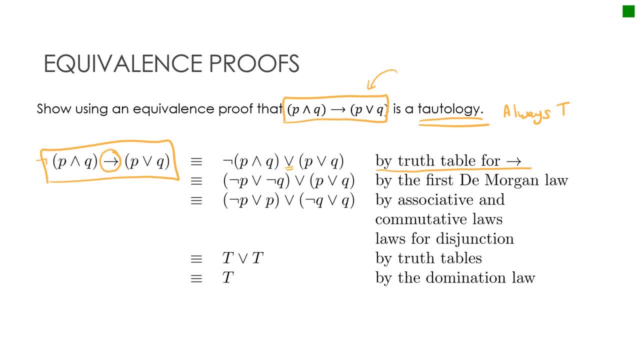 Then I'm using De Morgan's law, because I've got the negation of a compound proposition. So I'm negating each of those terms and switching it from a conjunction to a disjunction. Then I'm using the associative and commutative law. 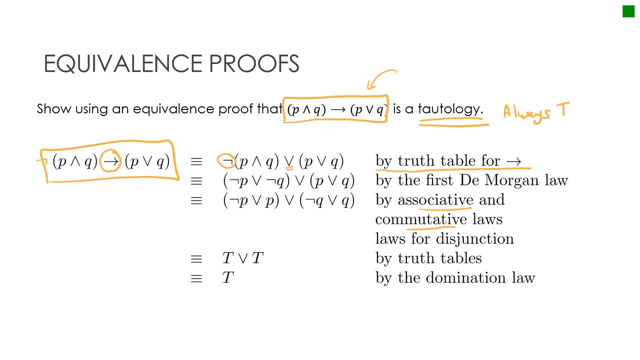 So, essentially, I'm switching the order and just grouping them differently. And again, I can do that because, notice, all of these signs are the same, Everything is the same. so I can use both of those laws And that gives me not P and P, which of course we know is true. 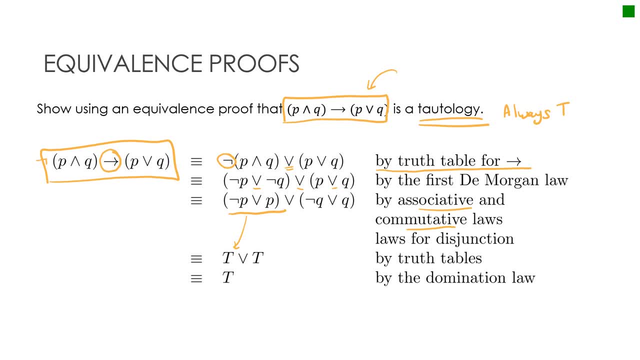 I'm sorry, not P or P, which of course we know is true, And not Q or Q. same idea, we know that's true. So now I have true or true, which of course is true, And because it's true, I've just proved that it's true. 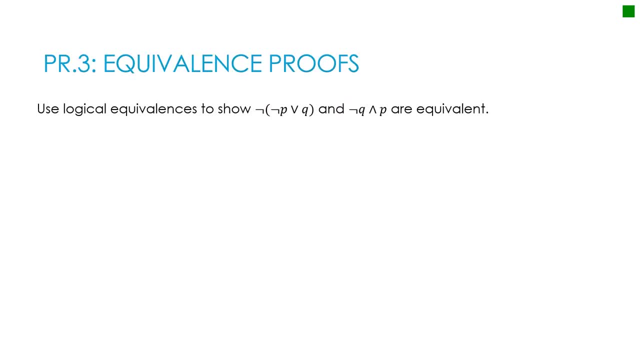 And that's why I'm using it as a totology. So now one of those for you to try on your own. So press pause, create your equivalence proof and then press play to see how you did. So this one wasn't so so bad. 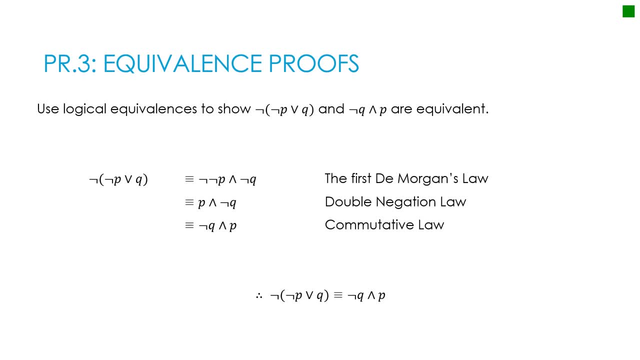 We started out with not or the negation of not P or Q, And I used De Morgan's law, as I do so often when I've got the negation of a compound proposition, And that gives me not, not P and not Q. 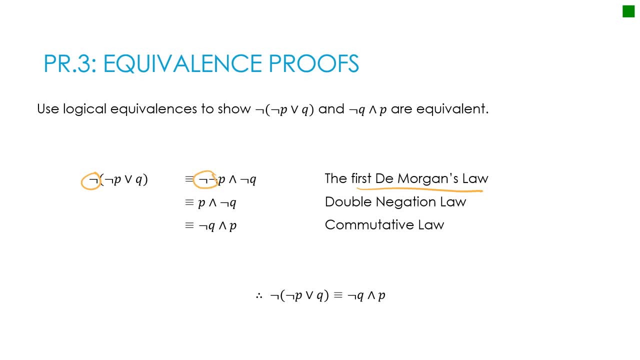 The not not P turns into P by the double negation law And then the commutative law says I can switch the order, And that's what I wanted is to end up right here. So hopefully you were able to arrive at that solution. 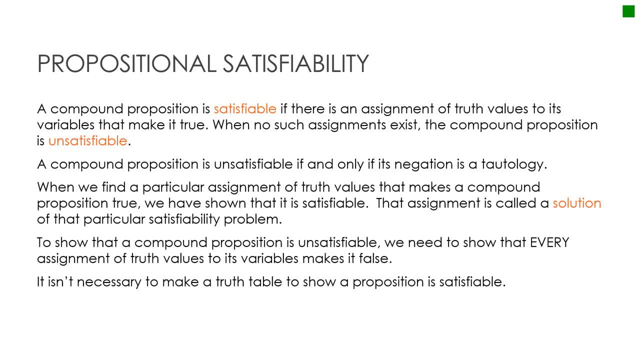 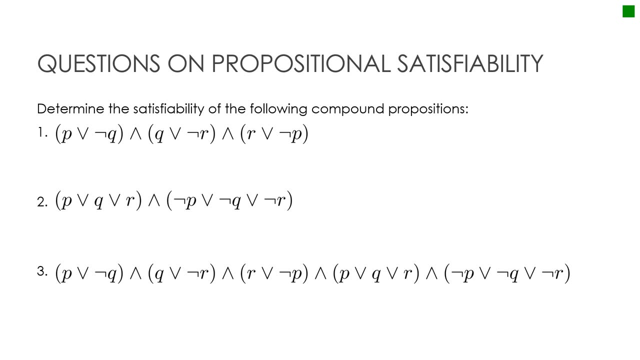 We're going to talk very briefly about propositional satisfiability. It's a little bit higher level or something that a lot of what. So we're going to look at a few examples of propositional satisfiability questions And essentially what we're doing is we're saying: 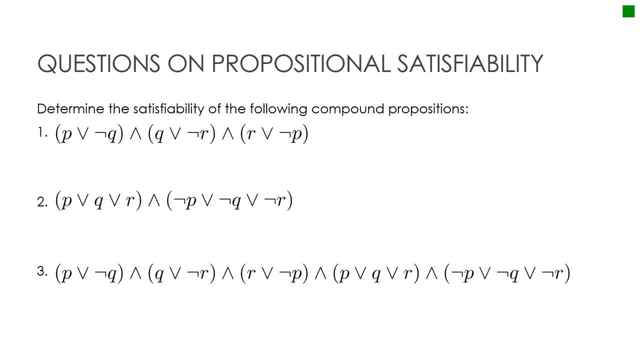 can we come up with some sort of truth value for P and Q and R so that this statement is true? We need the whole statement to be true. Now let's take a look at the statement. These are all ands And we know in an, and that means this has to be true, this has to be true and this has to be true. 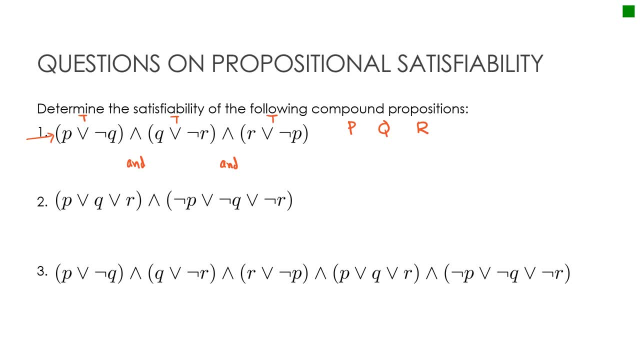 So it's really sort of a matter of reasoning combined with guesswork, Guess and check. So here let's make P true, Which means not P is false, And these are ors. So I just need one of those things to be true. 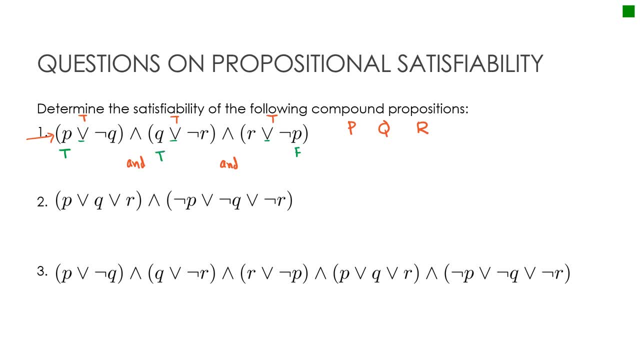 Well, what if I made Q true? Then not Q would be false, And that's okay. And here I'm going to need a true, So I'm going to put a true here and not R would be false. And so if P is true and Q is true and R is true, 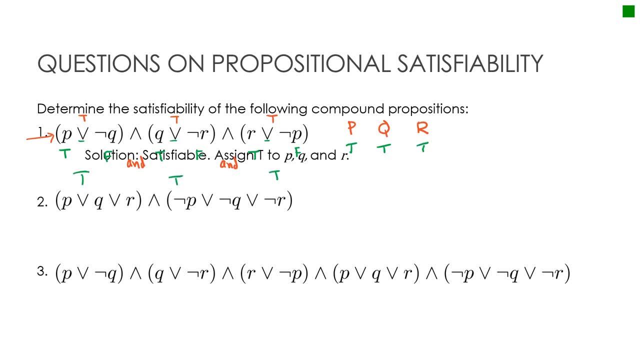 then I end up with exactly what I wanted: True and true and true, which makes this true. So if I use true for P and true for Q and true for R, it's satisfiable For to. again, I'm looking here at ands. 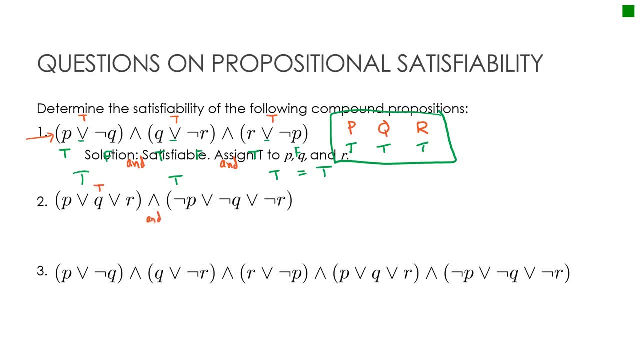 But all of these are ors, But ands tells me this all needs to be true and this all needs to be true. So it's not going to work for me To use what I did last time, which is true, true, true. 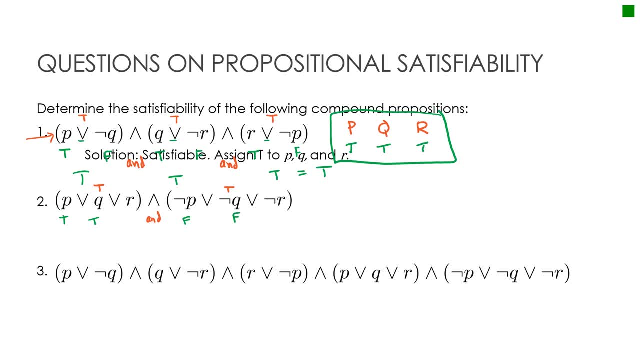 which would make this false, false. false because that would make this false and this true, And that's not what I want. I need them both to be true. So easy fix: Let's just assign R to be false, which means not R is true. 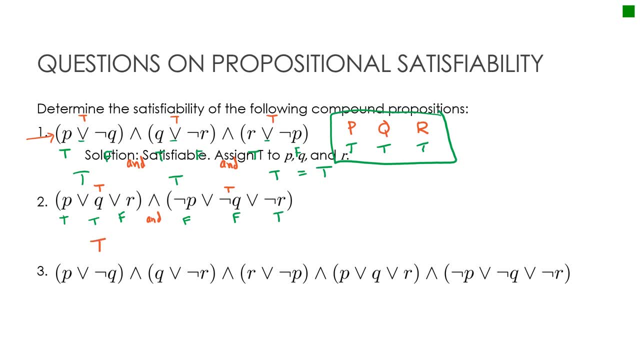 And now, all of the sudden, I end up with true here and true here. So there is one of the possible ways I make P True And Q true And R false, And that makes it satisfiable Again. if you came up with another way, that's great. 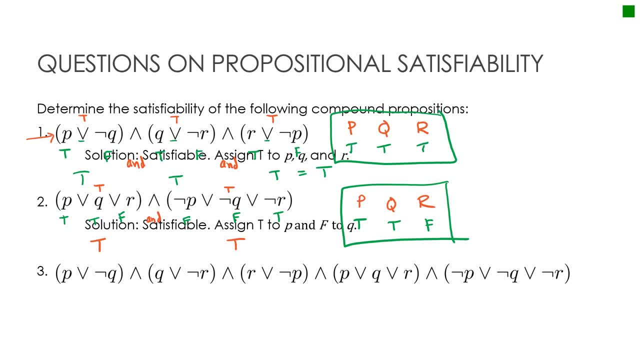 There's more than one way. So let's look at this last one. We've got all of these ands, which basically means all of these need to be true, Everything true, And this one obviously a little bit harder. But let's just start doing some practice. 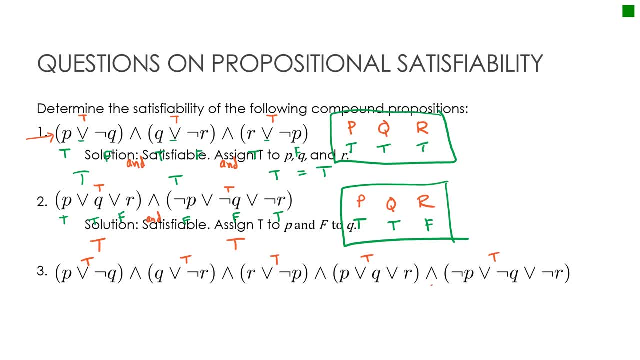 Let's say P Is false, which means not P is true. P is false, Not P is true. Well, that means I need not Q to be true in order for this to be true, which means Q is false, Q is false. 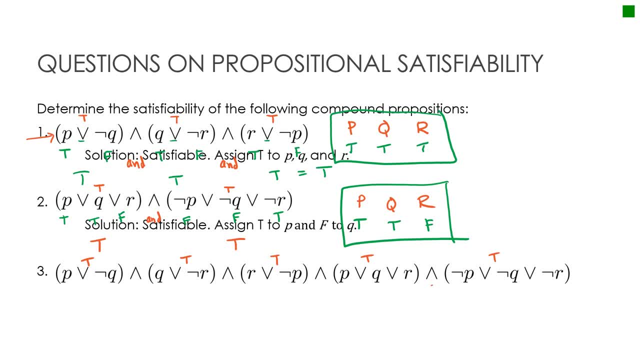 This is true. Now I need R to be true, Because otherwise this is not going to result in true. So if I make R true, then not R is false. So far, so good. Not R is sorry, R is true. 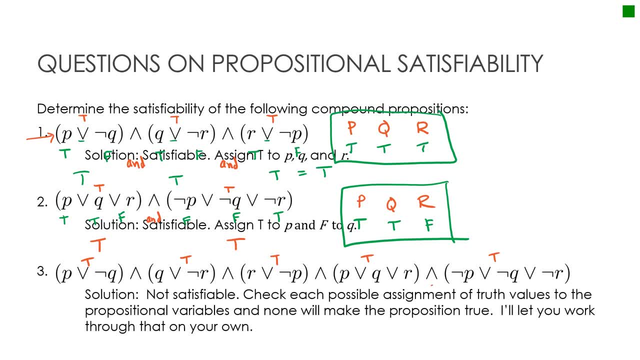 So that one's okay, But not R is false And we lost it right here. So it's impossible for me to make that work with P being false. But let's try it with P being true All the way back to the beginning. 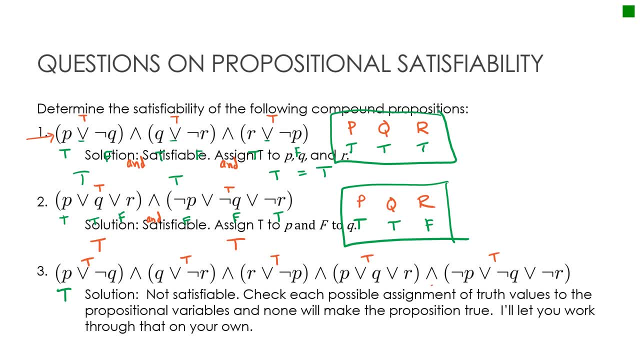 So let's say P was true, Not P is false. P is true, Not P is false. All right Then, if not P is false, R must be true. So R is true here. Not R is false. Not R is false. 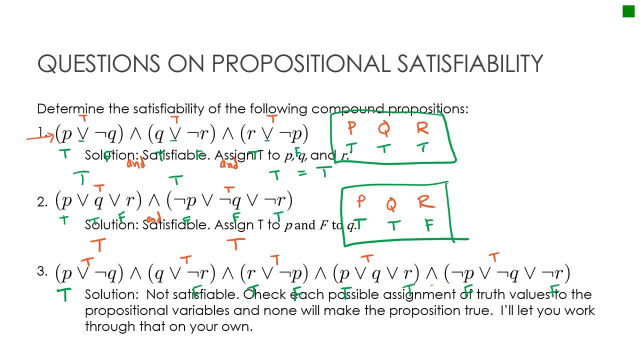 Here I would need Q to be true, So Q would be true, But that makes this false. And then I would need R to be true, But that makes this false And that makes this not work. So this last one actually is not satisfiable. 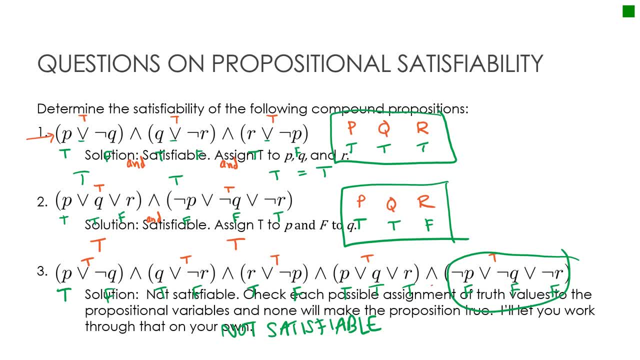 And again, the best way to do it is to make a truth table that shows all of the values and shows that it doesn't work. But we reasoned through that pretty well without a truth table, The next several slides I'm not going to spend a ton of time on. 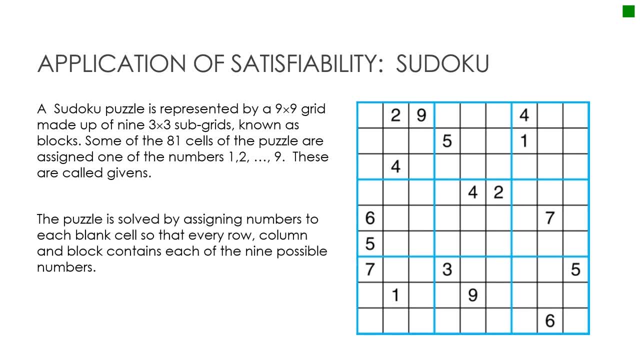 I just want you to know that there are applications of all of this. Obviously, a lot of this is, you know, a little bit more advanced than what we're able to do at this time, But Sudoku is a game that I certainly like to play. 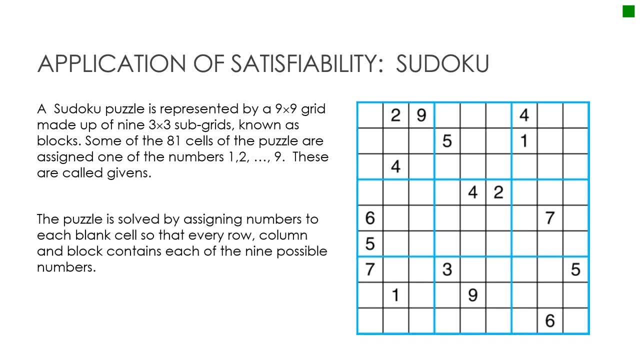 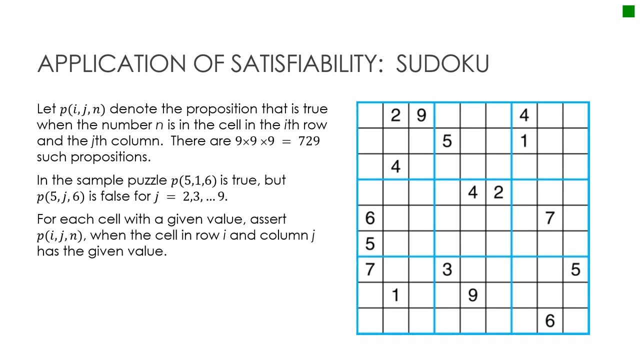 And, as hopefully you know, as Sudoku says that there has to be one of each in each row, one of each number in each column and one of each number in each block of nine. So if we're to do this using propositions p, i, j, n, where we can, let i be the row number, j be the column number and n be the number in the cell. 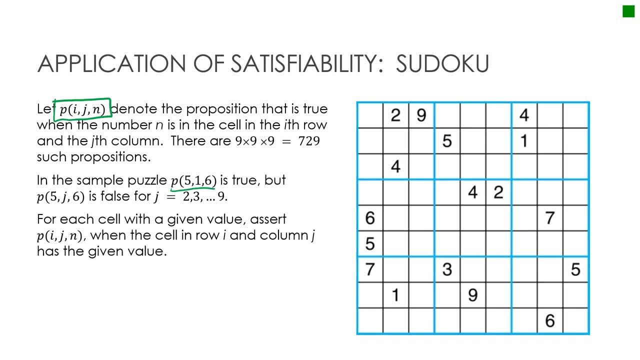 So p 5, 1,. 6 means row 5, column 1,, the value is 6.. But obviously it would be true. I'm sorry that would be true because 6 is there. But if I said p 5,, j 6, it would be false for 2 or 3 or 4 or 5, because obviously I'm not going to have 6 in any of those other numbers. 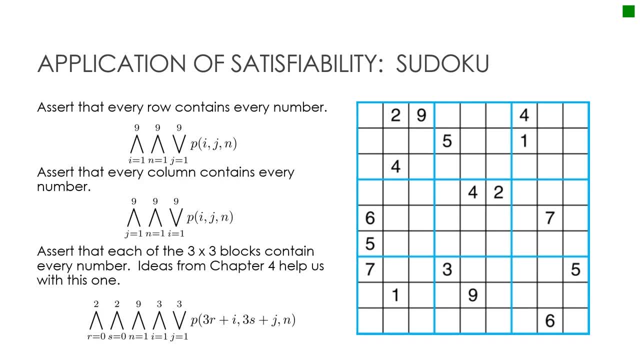 So, again going back to our sort of different notation that we talked about previously, We can assert that every row contains a number, That every row contains every number, which is what I've done here. Every column contains every number, And then this is far beyond the scope of what we know so far. 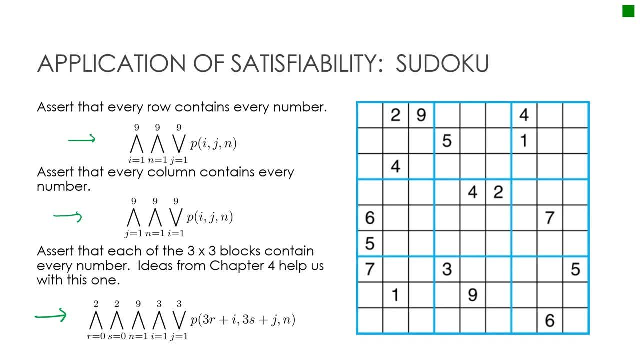 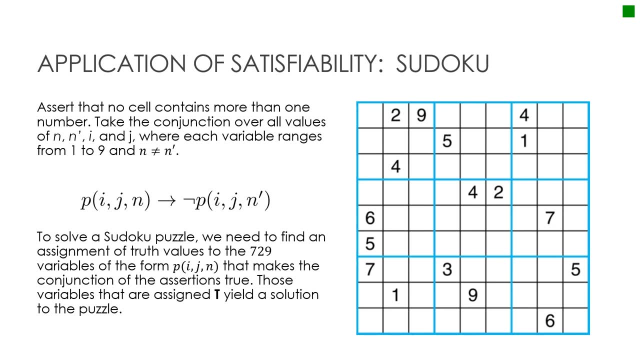 But that's what helps us to know that each 3 by 3 block has one of each number. Now there's no way for us to actually solve this based on what we know right now, But this just gives you an idea that this is how this might be set up mathematically. 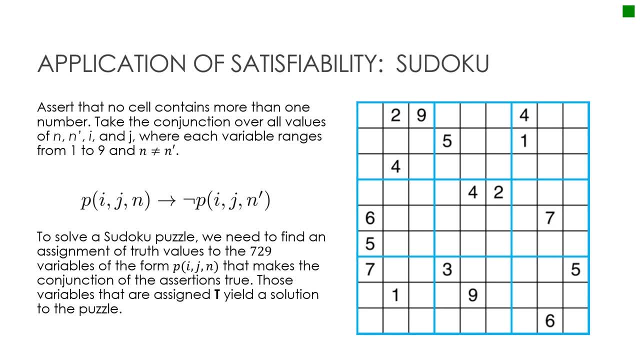 Remember that discrete math is very related to math. It's related to computer programming and such, And so something like this would be used in the creation of the program in order to solve a Sudoku puzzle, And those are out there all over the place. 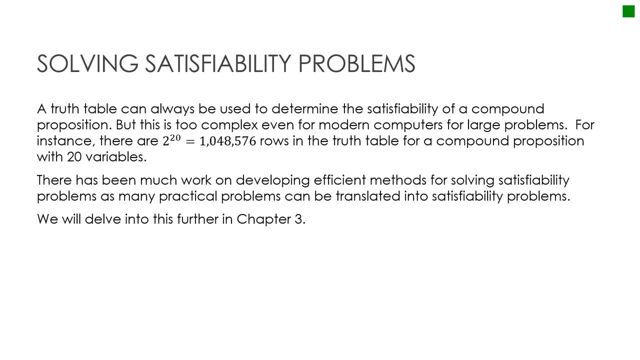 So essentially we can always use the truth table, But obviously it's going to be so much harder for a large compound proposition In this case. this is how many different rows of the truth table we would have to have in order to find something. 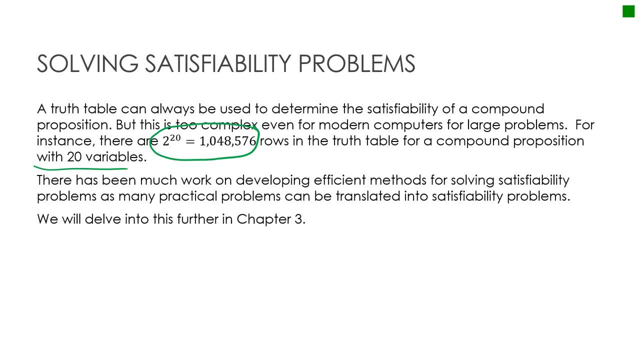 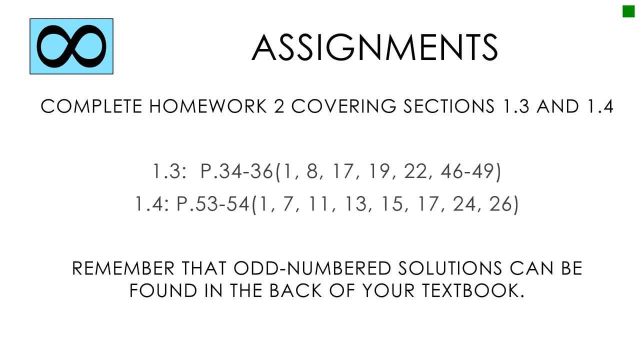 Even with 20 variables. We'll delve more into how to solve these in chapter 3.. But we're not going to get into the depth that would require us to solve the Sudoku puzzle. So your assignment 4,, 1, 3, and 1, 4 is given to you there. 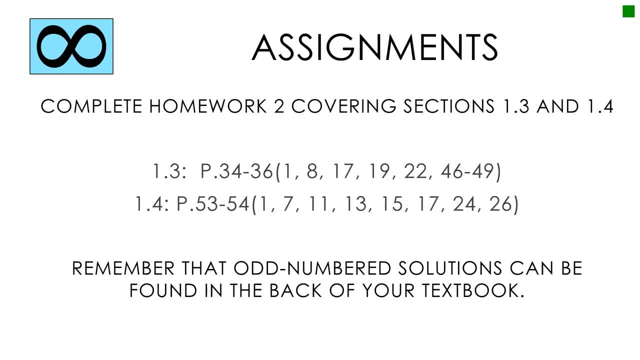 Remember, odd solutions are in the back of your textbook And I will see you in section 1.4.. 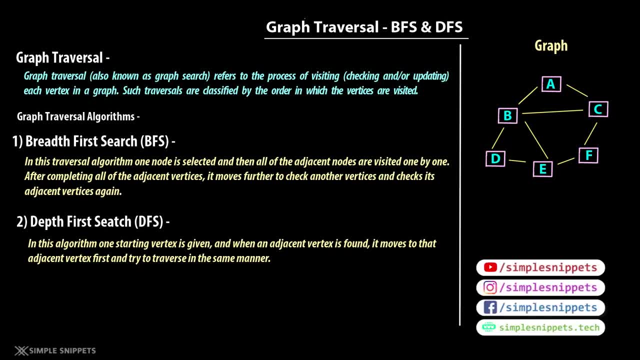 Hey, what's going on guys? Tanmay here for Simple Snippets and welcome back to another video tutorial on data structures and algorithms, And let's continue with our graph topic. We've covered quite a lot of details about graph data structure In case, if you're new on this channel, 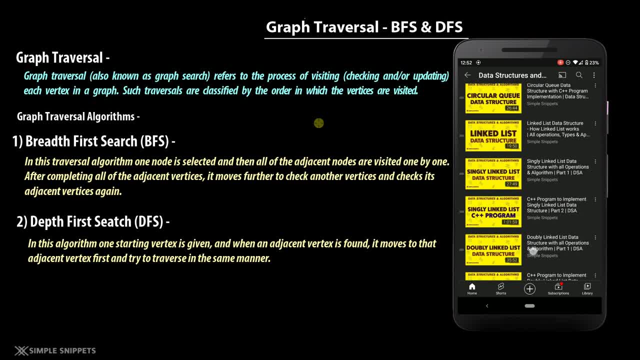 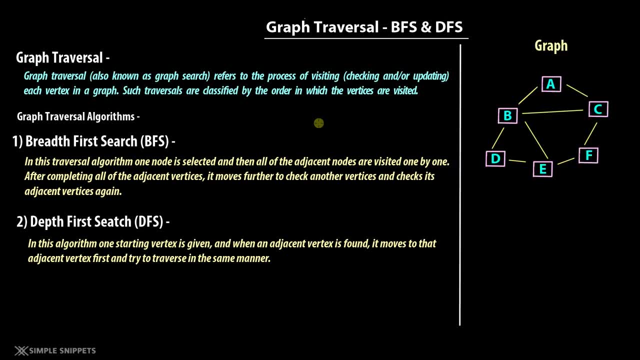 or, in case if you've missed the previous videos, check out the link in the video description to this entire playlist. Previously we've talked about what is a graph data structure, the theory about graph, how it is different from tree data structure, the different ways in which we can.